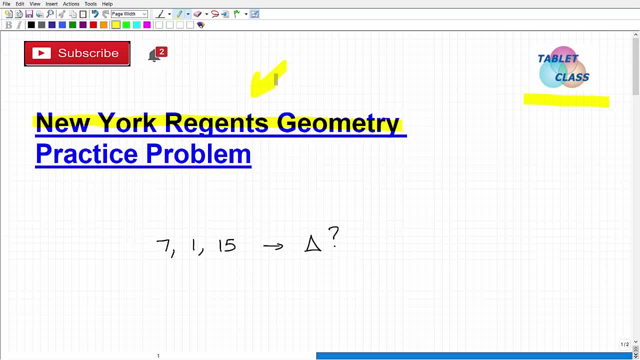 courses, to include a New York Regents geometry prep course. I'm going to leave a link in the description of this video. It's super comprehensive. Again, these are all courses that I've taught, And so if you're looking for some extra study, 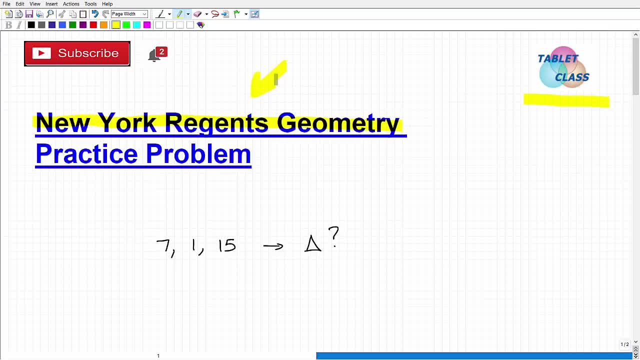 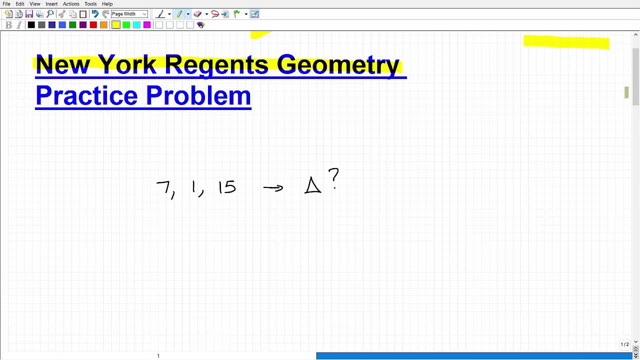 material. this course can definitely help you out, But let's get into this problem. Okay, And it's just basically a pop quiz, but it's something that you should be able to answer, you know, because it's an important topic in. 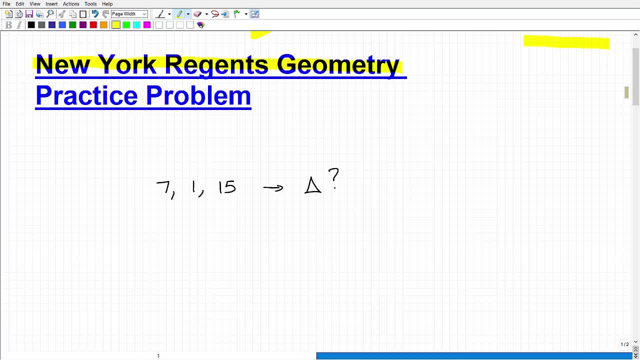 geometry Okay. So again you know, if you get this problem right, it doesn't mean that you're entirely ready for the New York Regents geometry exam. But if you get it wrong it doesn't mean that you know you're going to fail as well. Just 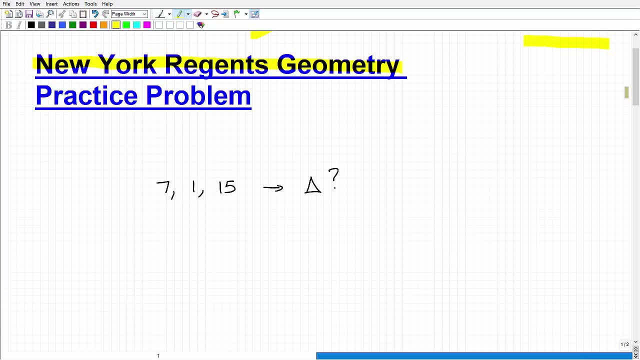 use it as feedback in terms of your preparation for this exam. Okay, So let me go ahead and tell you what the problem is, because this is just kind of like you know doesn't mean much, right here, Right, So here is what I want to say. Okay, So I 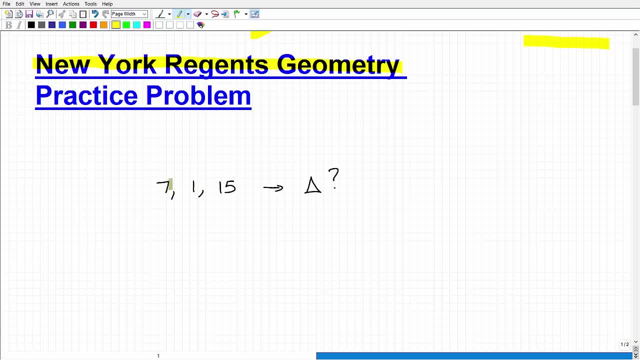 have three numbers here. I have seven, one and 15.. Okay, So I want to know if we can construct a triangle. Can a triangle be formed if the lengths of the sides of the triangle were seven, one and 15?? Okay, Is this an actual triangle? So in 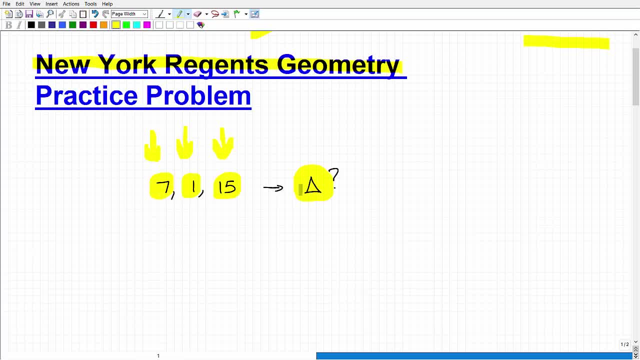 other words, is it possible to have a triangle with the lengths of seven, you know, seven inches, seven millimeters, whatever you want to think, one and 15. Use whatever units of measure you want. Okay, Now remember, we're going to be. 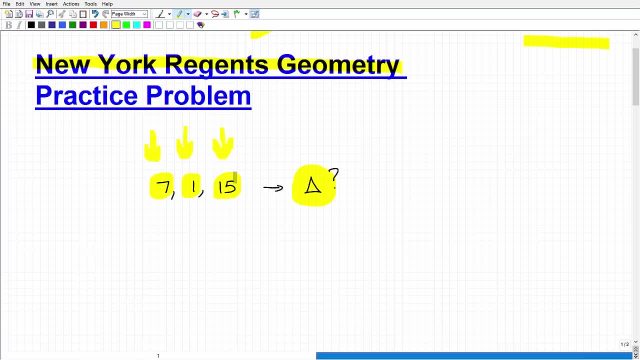 talking about the color of the triangle. We need to know what color the triangle is. We know what the color of the triangle is And we're going to be talking about the color of the triangle. What color does it have? Yeah, So now we're. 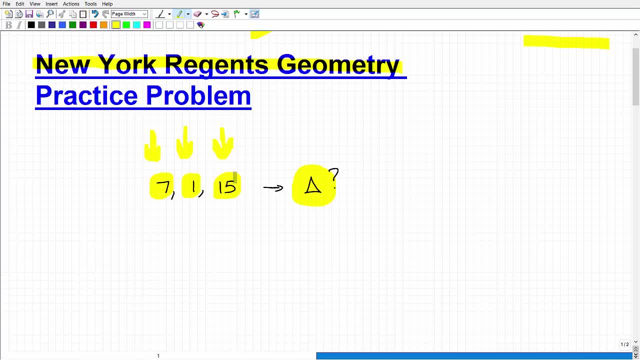 going to use our just a little bit of time and we're going to talk a little bit about our geometry. So when you're thinking about this problem, you need to be able to support your conclusions. So, uh, you know, if you're just kind of guessing you. know logically, if you want to kind of think about it, that's, you know good, That's fine. But you really want to think about what did you learn in geometry that really can support your conclusions to this answer? Okay, So you might want to go ahead. 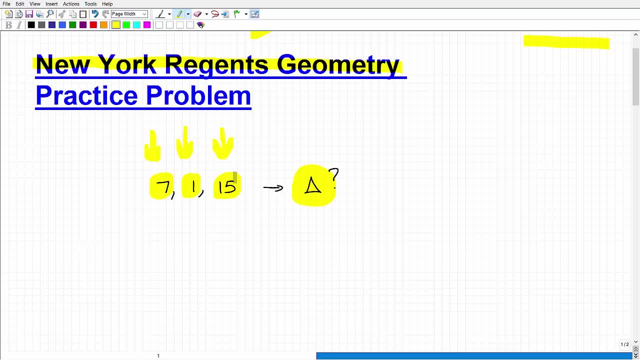 paused about a positive video and just thought about it and even if, uh, you're like i don't even know how to answer this, i'm just going to watch. the solution really should at least stop and kind of mess around with it. you know, just think about how could you answer this question. okay, so let's. 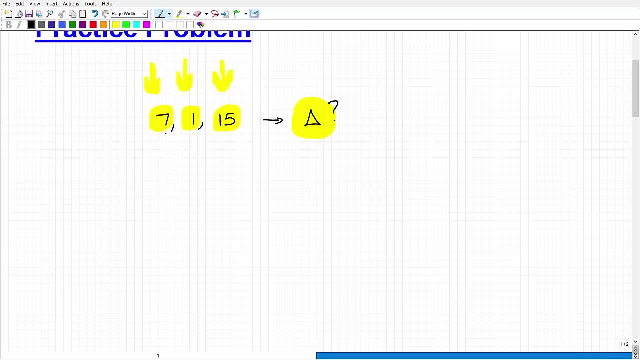 just take this approach. let's just kind of try to sketch a triangle of length 7, 1 and 15, so 15. that's pretty, you know, that's like twice, or more than twice, than this second longest leg of a triangle. so maybe it would look something like this, right? so let's say this is 15. so now i'm. 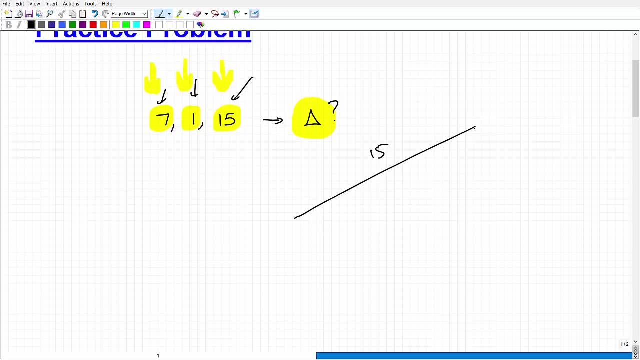 going to have one, a real short leg like: so maybe it's like that, all right one. and then i have seven over here. so now seven, i have to connect and form a triangle. but this is again, can only be- let me do it a little bit better- only be half of this 15 so you can see if i have seven. 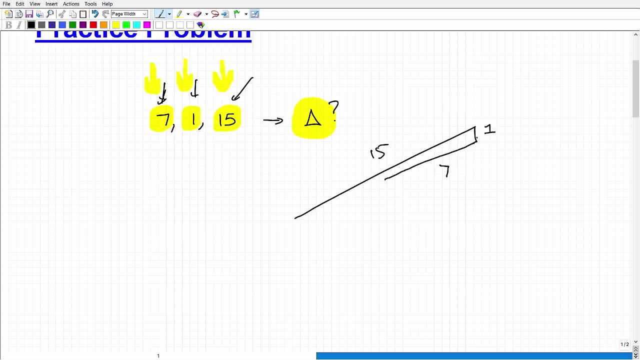 uh, that's, that's not going to work right. it doesn't look like we're going to be able to construct a triangle. so you're like, well, let's take this one and kind of scoot it over a little bit. so in other words, uh, let's make the angle more acute. maybe we can go like this one, just to kind of help that. 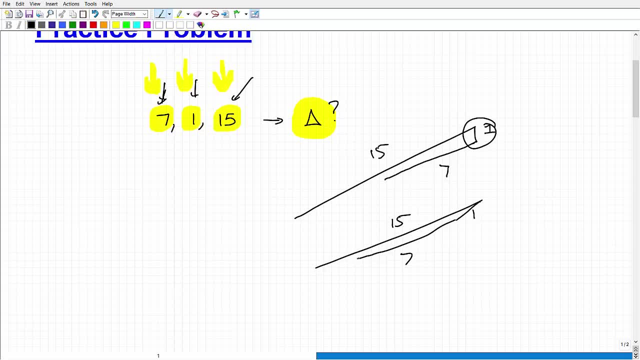 seven out, right? well, is that seven leg ever going to be able to connect to this, uh vertice or this, this point here at the end of this 15? well, no right, it's not going to be able to do that. so, from a common sense, uh, common sense standpoint, um, even if you don't know, 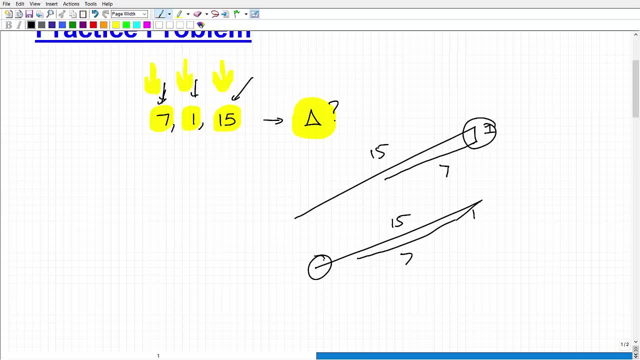 the concepts of why no? the answer, by the way, is no. we cannot form a triangle with these lengths. you can, kind of you know, always you know, before you give up on a math problem, you should always attempt it and try to use different kind of reasonings about it. but anyways, uh, this goes. 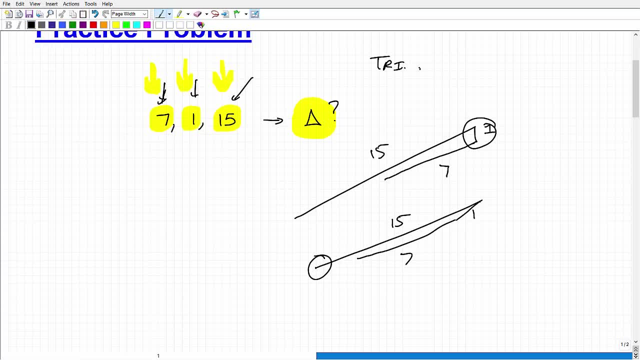 to something called the triangle inequality. okay, so you probably hopefully uh remember studying that. you definitely covered it, even if, uh, you don't remember it. it was kind of snuck in there in the course. but, um, there's uh triangle inequalities that have to do with lengths and 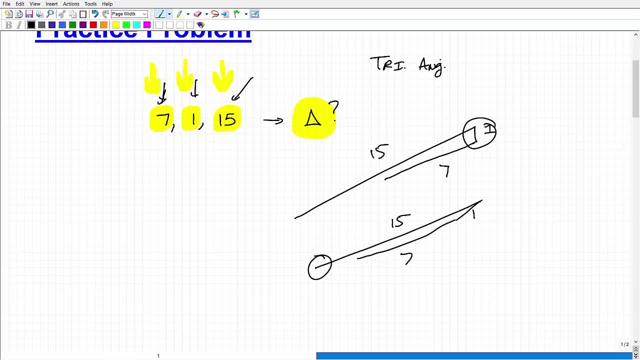 there's one that has to do with uh angles, but i'm not going to get into all of that. let's just focus in uh on here and the triangle quality. let's actually take a triangle that we know does exist, all right, and then i'll get back to why this can never be the lengths of a triangle. so we know that. 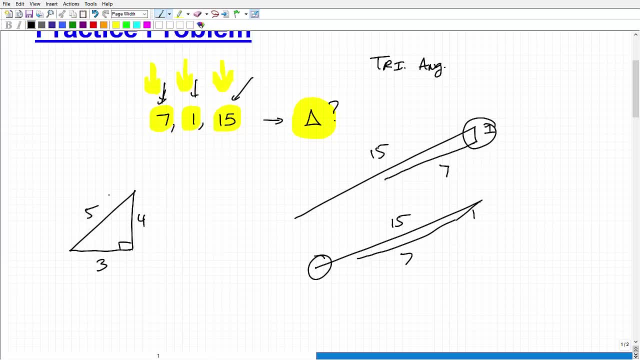 we can have three, four and five. okay, three, four and five. let me go ahead and erase this here. this is an actual triangle. it's a right triangle, it's a pythagorean triple. uh, so you should know that. but let's just go ahead and take a look at something. if i add up these two sides and two, 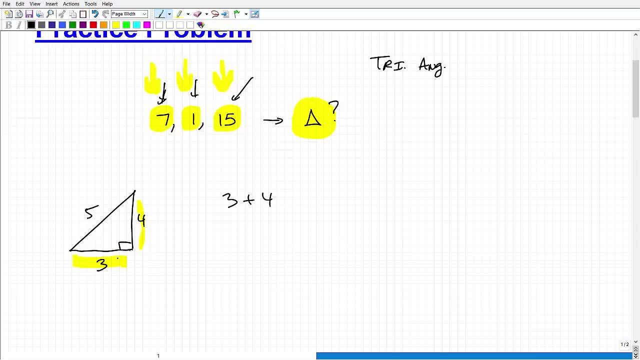 sides of a triangle, so it's three plus four. the sum of these two sides is going to be greater than this side. okay, right. so let's just go ahead and take a look at something. if i add up these two, three plus four, obviously that's seven. seven is greater than five. okay, now let's just go ahead. 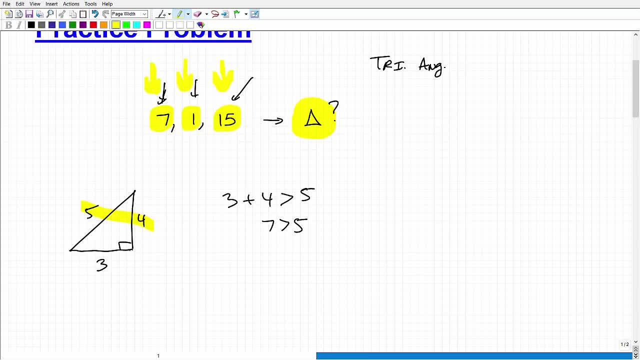 and add up any two sides of the triangle. let's do this: five and four. five plus four. is that greater than this other side? three, it is right, because that's nine. nine is greater than three. and whether there's uh sides, do we leave out five and three? okay, five plus three, all right, is that greater? 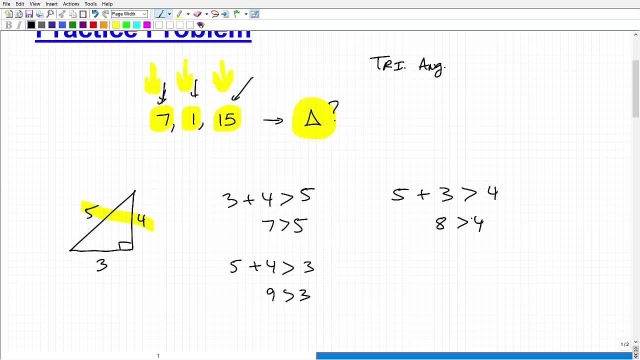 than four. that's eight. eight is greater than four. okay, so we did this combination as well, so you can see that any time. okay, we take two legs of a triangle. the sum- okay, that value is going to be larger than that third remaining leg. okay, so if 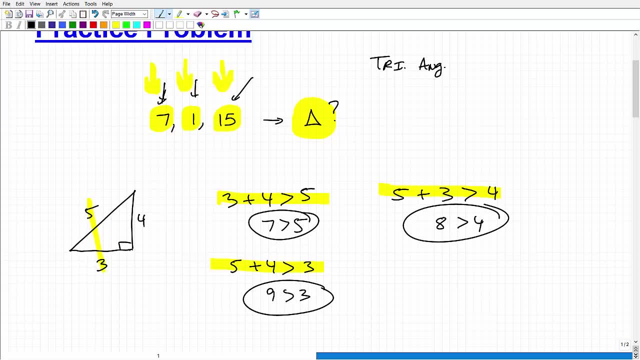 you have a triangle, okay, you will always have this uh condition: okay, this is always going to be true. so that's why this scenario: okay, without even trying to sketch it out, it's not going to work, because let's just kind of, uh, do the same thing with these lengths, okay, so we have 15 plus one. 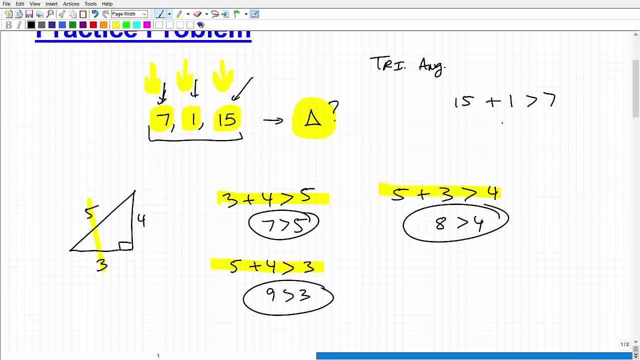 is that greater than seven? yes, that's true, right, 16 is greater than seven. that works. is 15 plus seven greater than one? obviously that's true as well. okay, so true and true. but now we run into problems by seven plus one. is seven plus one greater than 15? no, eight is not. 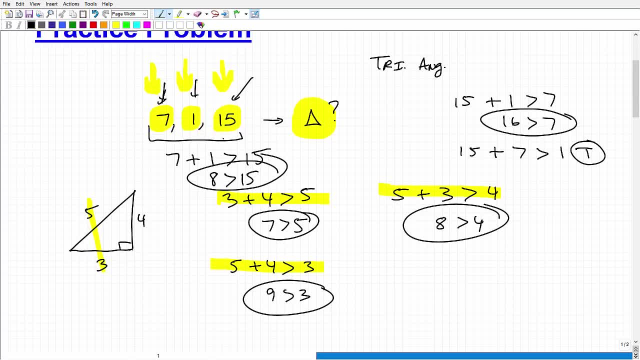 greater than seven, greater than one. okay, so that's true, but now we run into problems by seven plus one is that greater than seven is less than 15? ignore the eight. remember we ran into problems by seven plus one is smaller than five. okay, and that is what we're. 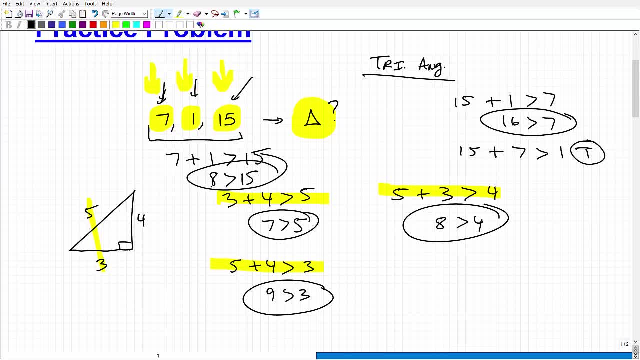 planning on, okay, and let's look at how we can accomplish that now. let's look here. there's five elements, okay. the behind it looks like this is a left axis and that's it's. this is a right axis, and we're running into a right axis here and we're fazendo some of these arrangements, okay. 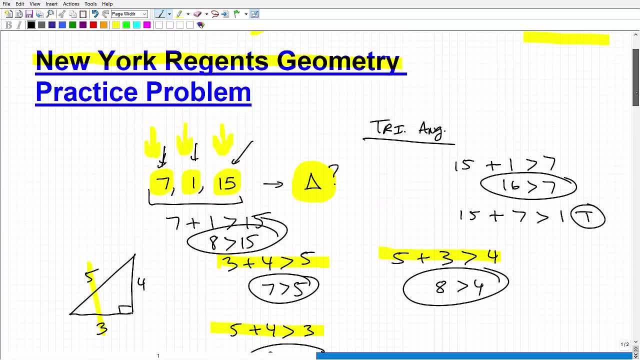 now. so what we're going to do is we're going to highlight a first ingredient. we're going to- i'm not calling this the final part of the equation. you want to just do the final part of this as a calculator of what we found: the right three Nederlanders that we found on the right. 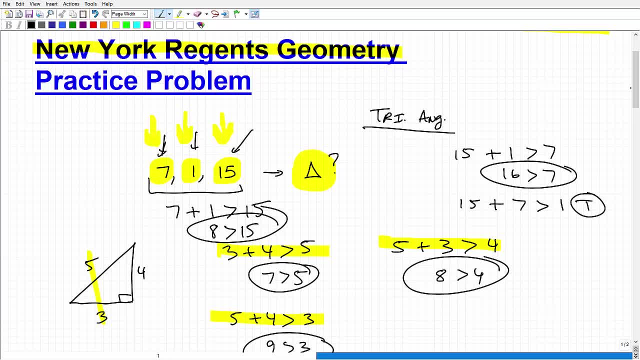 field, okay, so give us yourettuland zero. we have l two to Oneabs and let's just say two vers sık. the quality is or even like it's a theorem or a postulate or an axiom. you know, you got to remember the, the concepts, okay, so don't try to just use rote memorization and look at it especially. 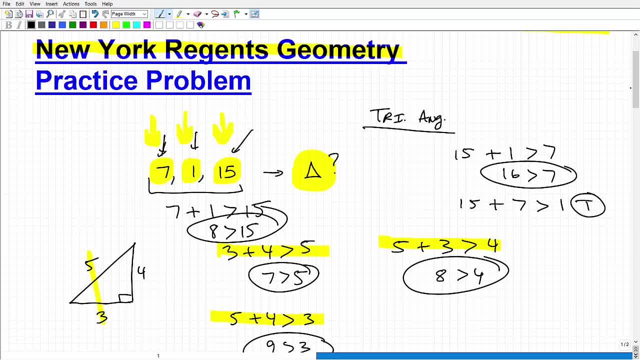 when geometry. geometry is one of those subjects that you know. you're flooded with. you know postulates and theorems and and there's things, corollaries, lemmas, i mean it can go on and on. there's a huge amount of information. your teacher doesn't expect you to know it. you know the rote. 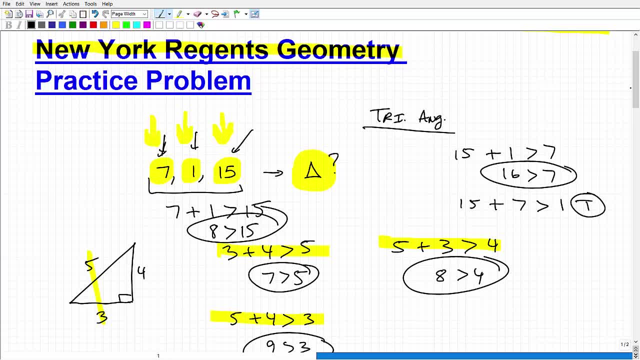 you know, in other words, like to write it down perfectly. the main idea is the concepts. okay, do you remember the concepts? right and um? a triangle. inequality is something you definitely want to know. uh, and you know, this is something that you can definitely see on the region exams important. 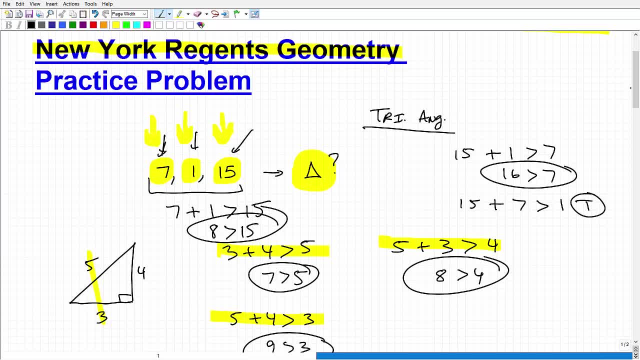 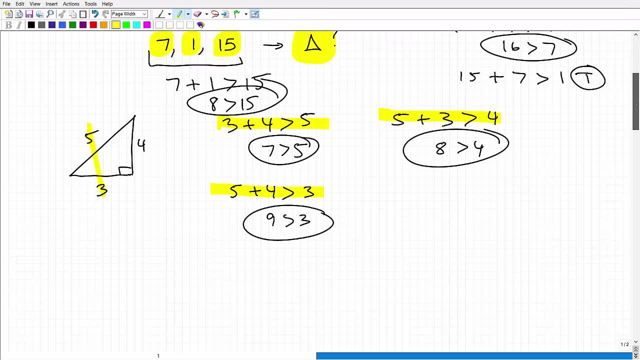 this comes up, uh, even in other type of standardized tests that you might see, like sat, act, etc. okay, so let's go ahead and wrap up this video. again, it's not gonna be a full lesson on the triangle inequality- again, we can talk about angles, etc. but 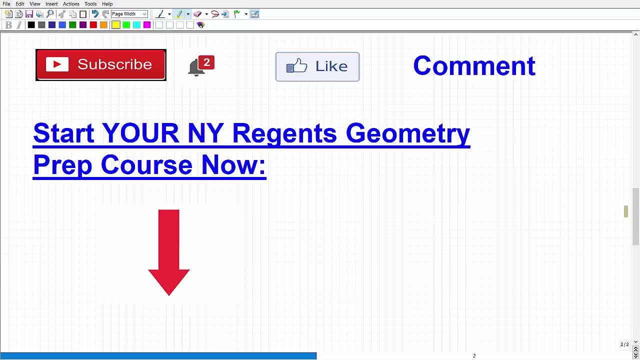 it's something that hopefully, uh, you remember covering in your course. if you haven't, definitely you know you need to kind of go back and study. but i can almost guarantee you that you- uh, you know, definitely covered it, but it's one of those smaller topic that sometimes students